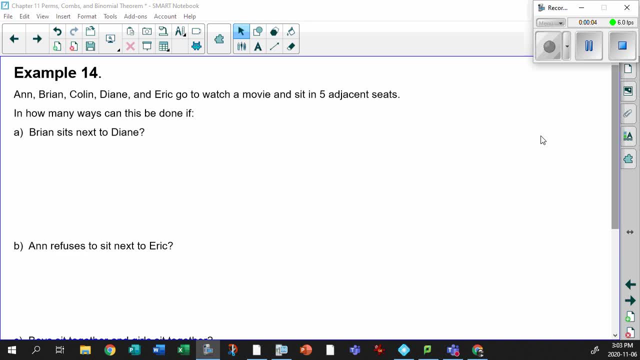 Here's the last question. we're going to do with fundamental counting principle and some really nasty conditions. Okay, so we got Anne, Brian, Colin, Diane and Eric- five friends going to watch a movie and they're going to sit all next to each other while they're. 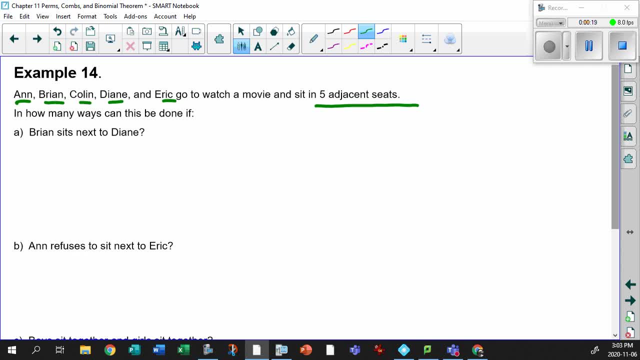 watching this. But now let's throw the conditions on here. The conditions are: oh, guess what? Oh, Brian wants to sit next to Diane. Oh, they must be dating. Oh, it's so sweet. Okay, stop, All right. so Brian has to sit next to Diane. So think about it. You have two possibilities here. 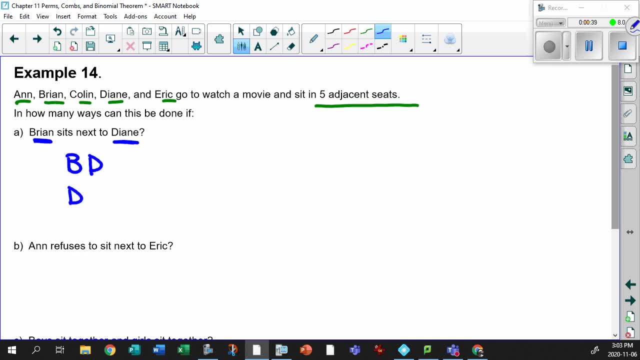 You have Brian that can sit first and then Diane, or you can go Diane and then finally it's Brian. So if you think about it out of this, you have two possibilities for that. Oh, that's interesting. So every time Brian and Diane show up, they have two possibilities. 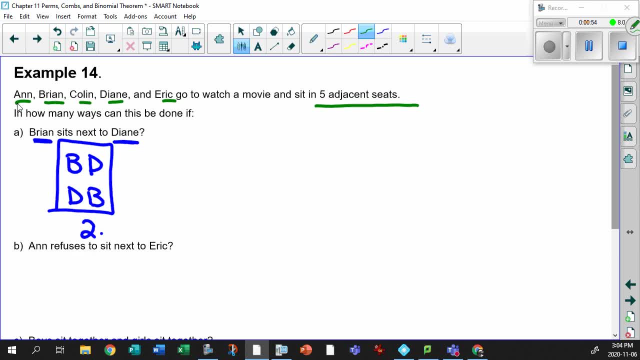 So my next question is: what is the most important thing to me? My next question, then, is: what else do we have left? If we dealt with two people and we have five friends, we have three people left that we have to deal with, right? So if you think about 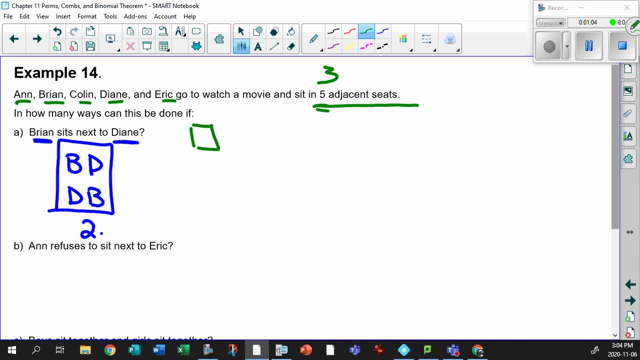 it. Brian and Diane could be in the first seat right here right, Or the first two seats. There's Brian and Diane in the first two seats. Then think about it: One of the three friends can be here, followed by another friend, followed finally by the last friend sitting in that. 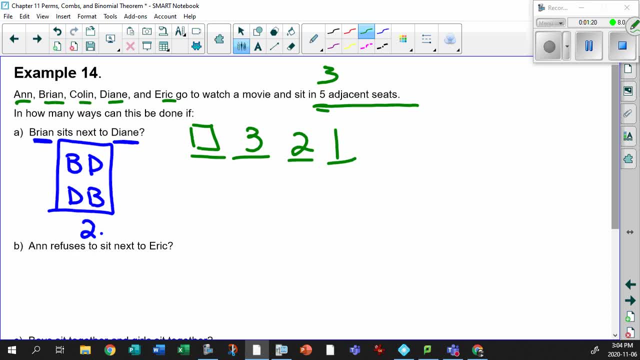 arrangement. So Brian and Diane can be up front and remember there were two possibilities For their arrangement: Brian and Diane or Diane and Brian. okay, But what if Brian and Diane want to sit one seat over? So that means they want to sit here. okay? Well, you still have Brian and Diane. 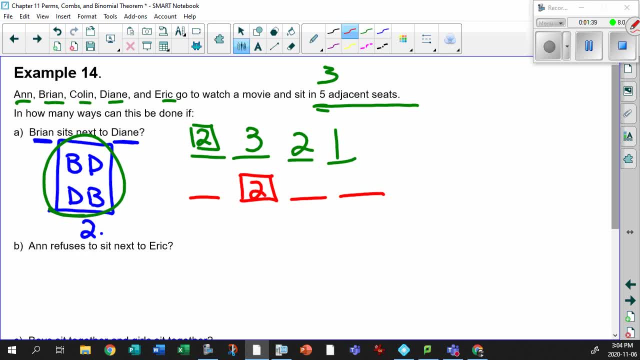 That's still two possibilities there, right? Either Brian and Diane, or Diane and then Brian. And then you still have three choices for this one, two choices for that one and one choice for that one. Watch again now, because Brian and Diane are going to move again. Oh, they're just never. 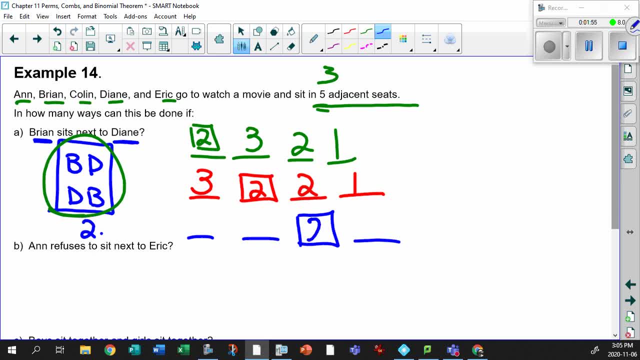 happy unless they're moving. There we go. So we have two choices for them, right? So three choices for the first seat, two choices for the next seat, one choice for the last seat And then, finally, the last arrangement we can have again is Brian and Diane at the end. Now they're way over on the 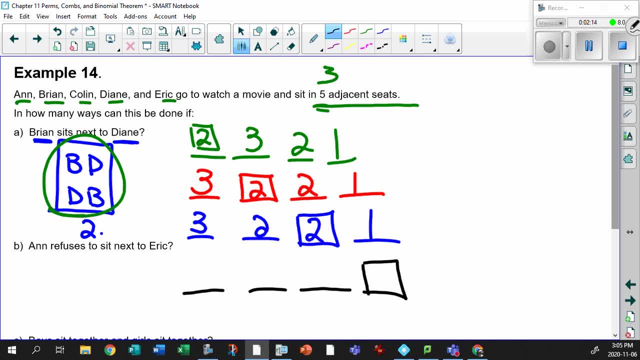 right side of the of the row. Okay, whatever. So you still have three choices here. two choices here, one choice for here and, of course, two choices for Brian and Diane. and Brian. Now multiply these guys out. When you multiply these guys out, think about it Two times: three is six. 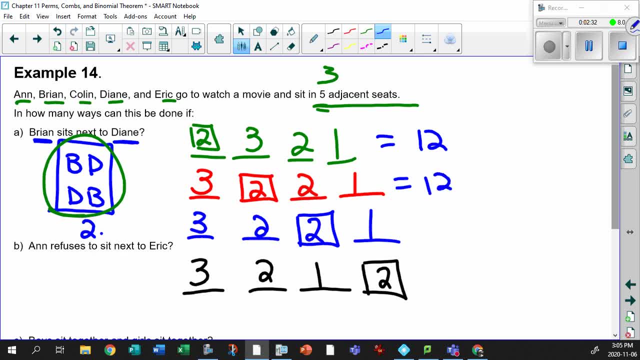 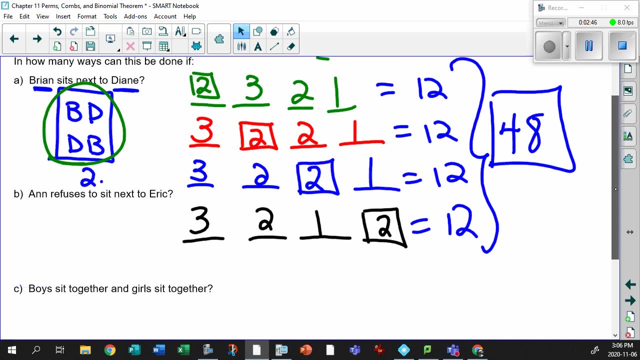 times two. You've got 12 arrangements here, you've got 12 arrangements here, 12 arrangements here and 12 arrangements here, For a total of 48 possible arrangements. Yippee, skippy. Now let's take a look at one more kind of rendition: Very, very similar, Very very similar. 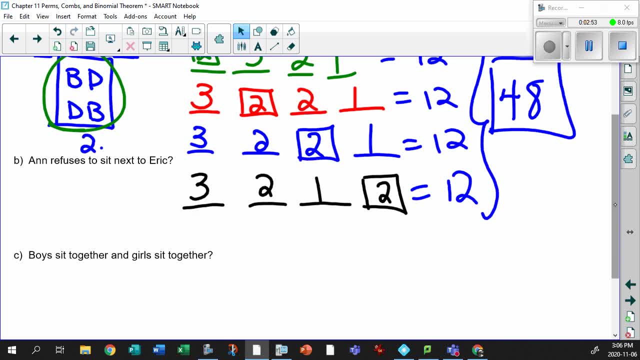 Think about this: Anne refuses to sit next to Eric. Well, how do we go about doing this? Do we start putting Anne one here and then choices for the other ones, and so on and so forth? Well, you could, or you can, use something called watch. this, it's called the complement. Okay, so, in other words, start with. 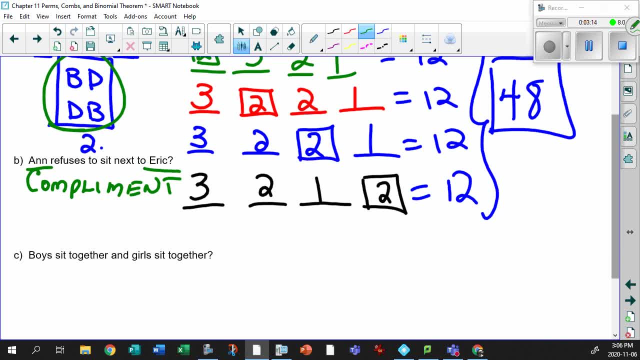 Anne sitting next to Eric. Start with Anne sitting next to Eric and go through all the possibilities. Well, guess what We just did? We did it right here With Brian and Diane. Now we'll do the exact same thing with Anne and Eric and say yes. 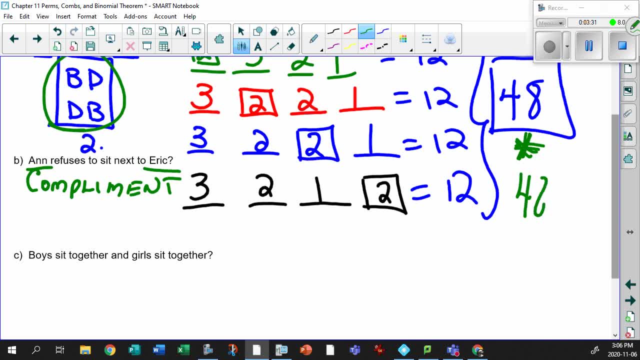 let's force them to sit together. So that means we have 48 arrangements of them sitting together. Okay, Sitting together. There we go. Okay, We have 48 arrangements of that, But wait a second, We're told we don't want that. So that's a negative thing, isn't it? 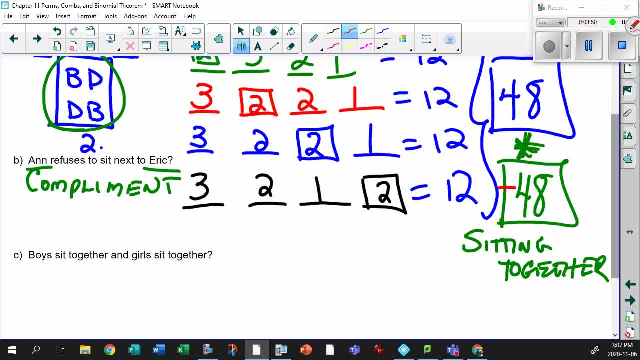 That's an awful thing, That's a negative. Well, great, You know. what we can do Is let's figure out how many arrangements there are of everybody. Think about it: You've got five people at the theater: One, two, three, four, five. We've got five possible seats, So five choices for. 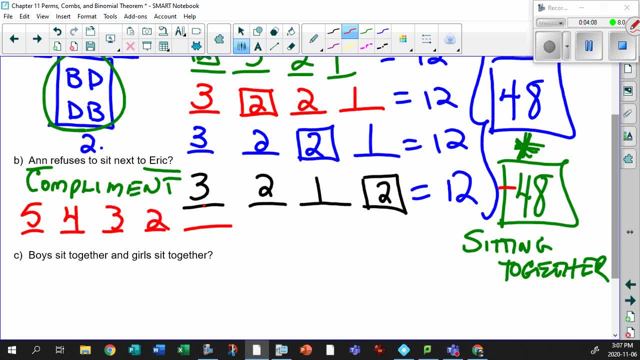 the first one, Four, three, two, one, And if you multiply all that together you get a really nice number of 120.. That's all the possible arrangements. But now what we're going to say is: we don't want this. 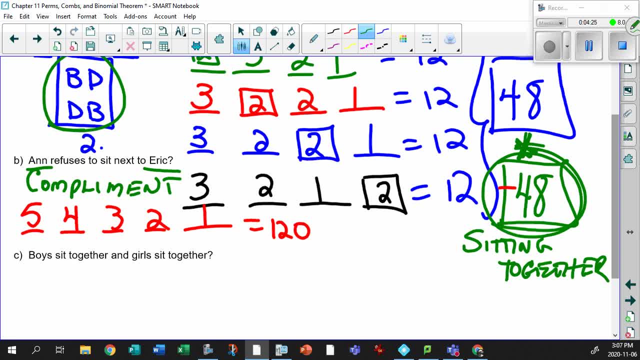 We don't want them together, but we know that there's 48 arrangements of that. Oh, okay, So that means I'm going to subtract the ones that I don't want. That's called the compliment. So if you subtract that out, you end up having 72 possible arrangements. 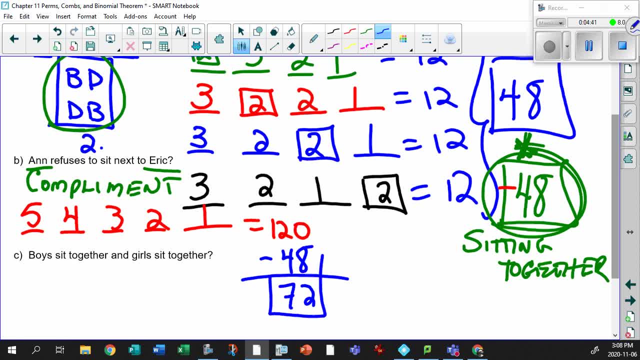 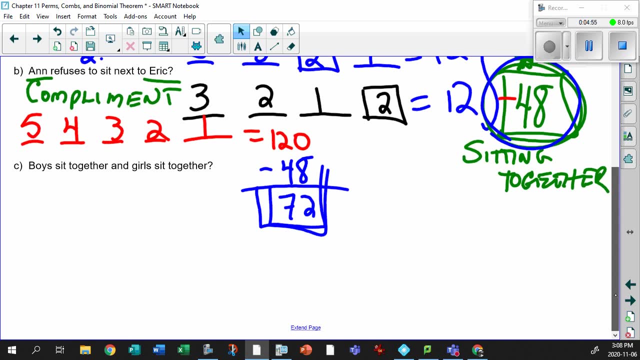 where Anne and Eric are not sitting together. You see how it works. You put them together first, subtract it from the total and you get what's left, which is 72 arrangements. Oh, that's just two, Sweet Okay, Now, last one that we have to figure out. The last one is this one: Boys must sit. 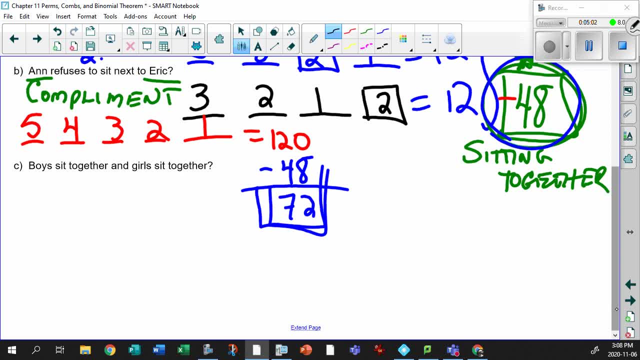 together and girls must sit together, And we've done something similar to this before. So if the boys sit together, they're all going to sit on one side. There's the boys, Girls sit together, There's a girl sitting on another side. Okay, Let's figure out how many boys we have and how many girls we 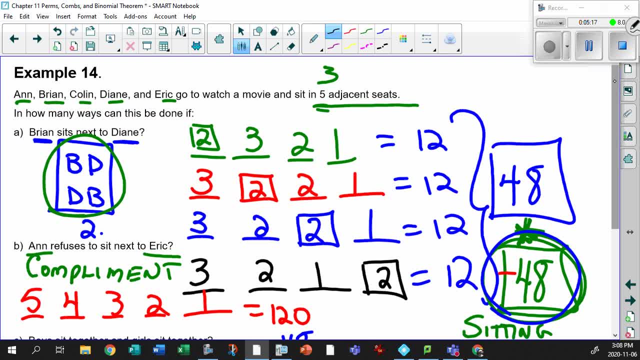 have. Let's go back to the top Right. So we have Anne, that's a girl. We have Diane, that's a girl, And that's it. So we have two girls. That must mean three boys, Sure enough, Brian Colin. 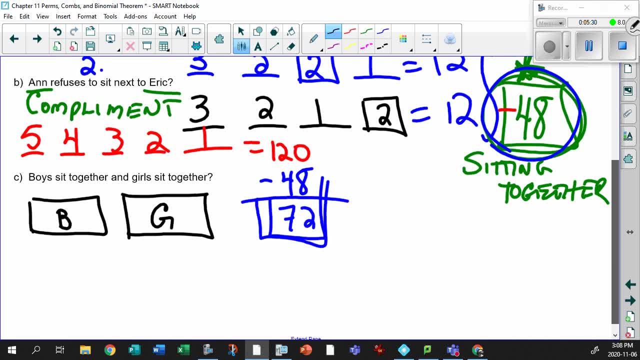 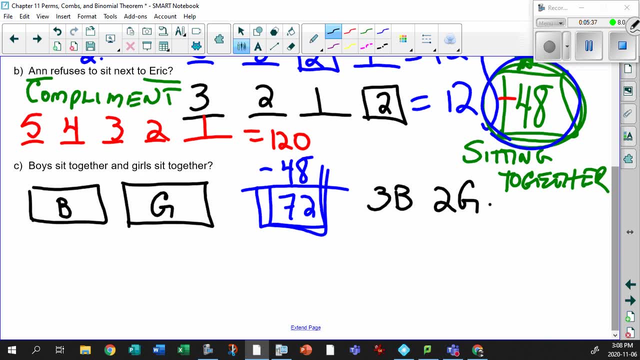 and Eric. Two girls, three boys. Okay, Let's answer the question: Two girls and three boys. There's three boys, There's two girls. Let's go to town, Okay. So how many arrangements of boys can we have? if we sit the boys on the left-hand side? Well, first chair would contain three. 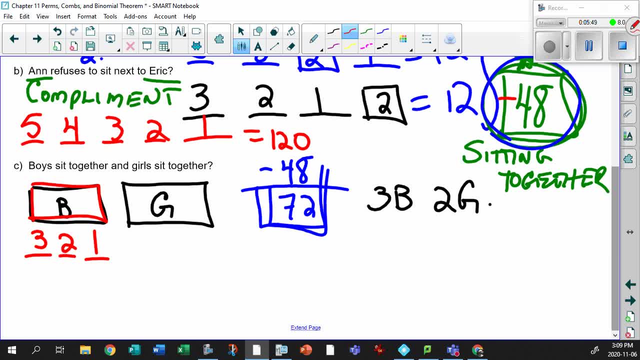 The second chair would contain two and one choice for the third chair. On the girl's side, we have two choices for the first chair, one choice for the next chair Makes sense. Okay, How about if we flip this around? Well, wait a second. Three times two is. 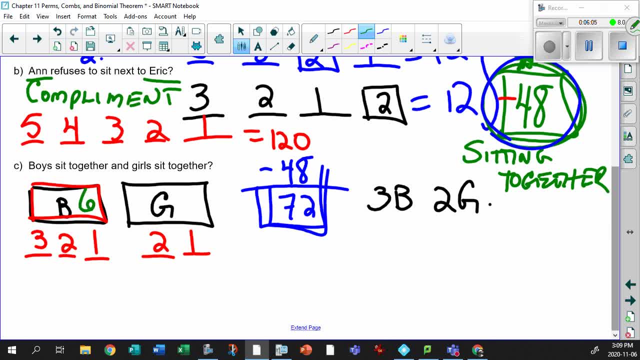 six times one. That's, of course, six choices for that. Two times one. we have two choices for that. Oh, yippy skippy, Six times two. we have 12 arrangements. if they sit, boys on the left, girls on the right. But I'm also curious then is what if the girls are on the left and the boys are? 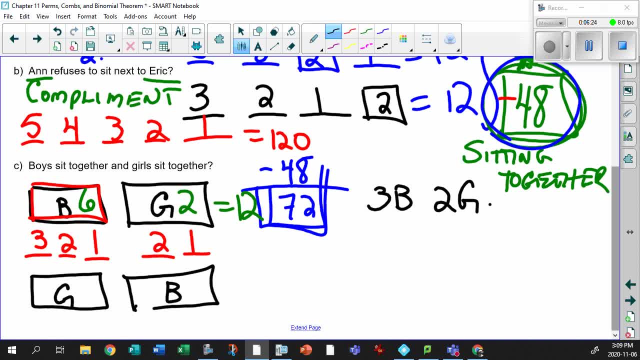 on the right. Well, the arrangements don't change. There's still for the girls, only two arrangements for the girls, And of course there's six arrangements for the boys. So two times six also gives you 12.. I got a question. Is this an and or an or? Hmm, Think about it, You can. 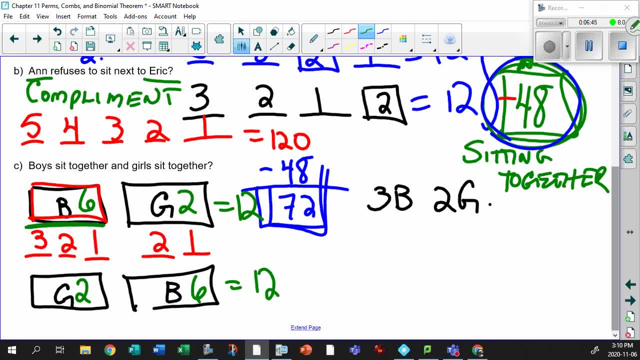 have the boys on the left or the boys on the right, which means you add this, So a total of um 24 arrangements. Wow, That was cool. Stay tuned. More stuff coming up, including perms, comms and factorial notation. 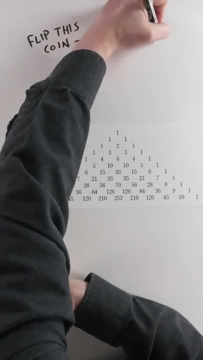 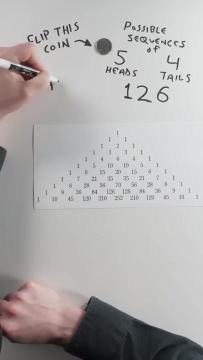 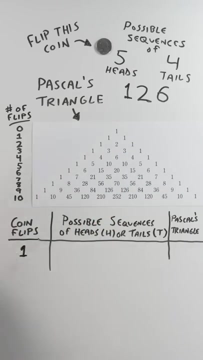 If I flip this coin nine times, I can tell you exactly how many possible sequences of five heads and four tails exist: 126, because I've got Pascal's triangle. Consider each row to be the number of flips. Top row is zero. next row is one coin flip with two. 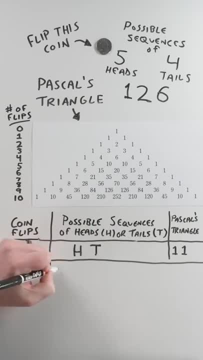 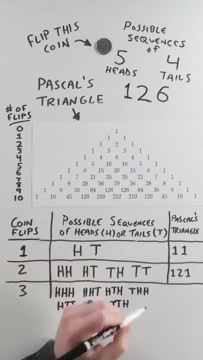 possible outcomes: head and tail. With two coin flips you can get four possible results: Head, head, head, tail, tail, head, tail, tail And three flips looks like this: So nine coin flips can result in one outcome of all heads, nine different outcomes of one head. 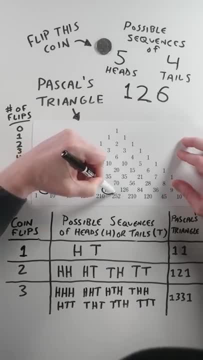 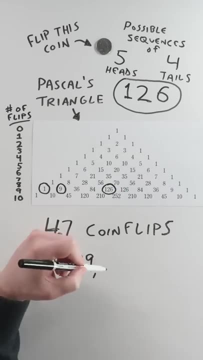 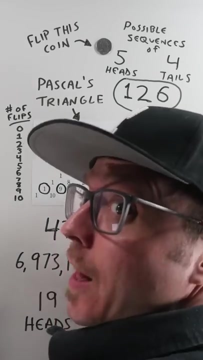 and eight tails, all the way to 126 outcomes of five heads and four tails. 47 coin flips generate 6,973,199,770,790 possible arrangements of 19 heads and 28 tails. Now you know that, Okay, bye.